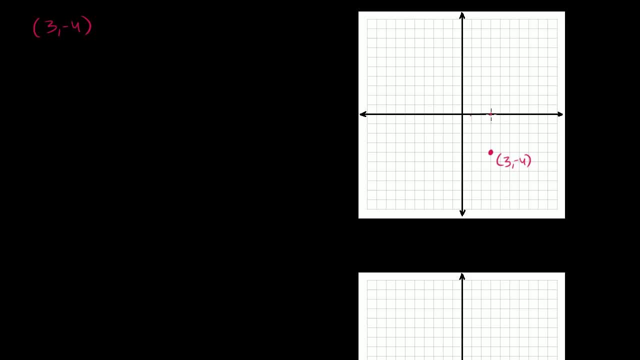 And I also have the point 6, comma 1.. So 1,, 2,, 3,, 4,, 5,, 6 comma 1.. So just like that, 6 comma 1.. In the last video we figured out that we could just use the. 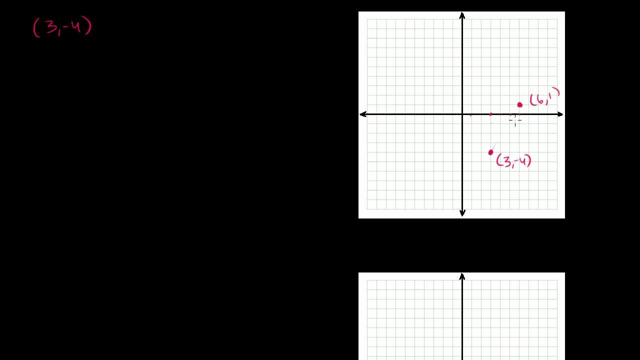 Pythagorean theorem. if we wanted to figure out the distance between these two points, We just drew a triangle there and realized that this was the hypotenuse. In this video we're going to try to figure out what is the coordinate of the point that is exactly halfway between this. 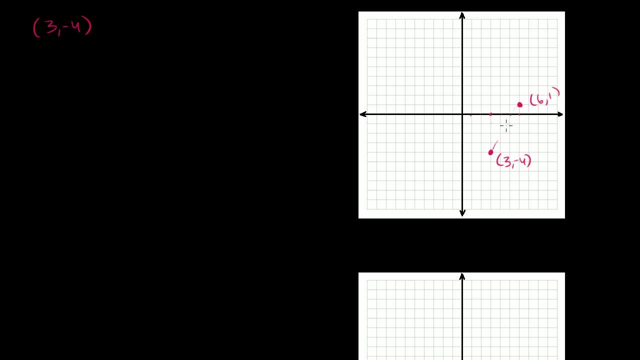 point and that point. So this right here is kind of the distance, the line that connects them. Now, what is the coordinate of the point that is exactly halfway in between the two? What is this coordinate Right Right here? It's something, comma, something. 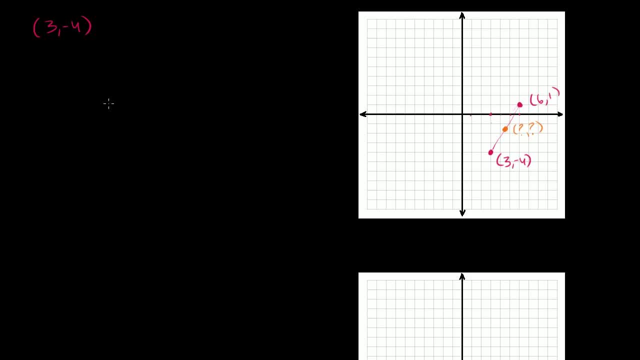 And to do that, let me draw it really big here, Because I think you're going to find out that it's actually pretty straightforward. At first it seems like a really tough problem. Gee, let me use the distance formula with some variables. 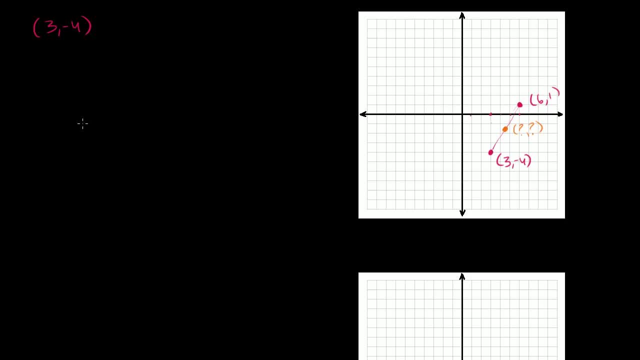 But you're going to see, it's actually one of the simplest things you'll learn in algebra and geometry. So let's say that this is my triangle, right there. This right here is the point 6, comma 1.. This down here is the point 3, comma negative 4.. 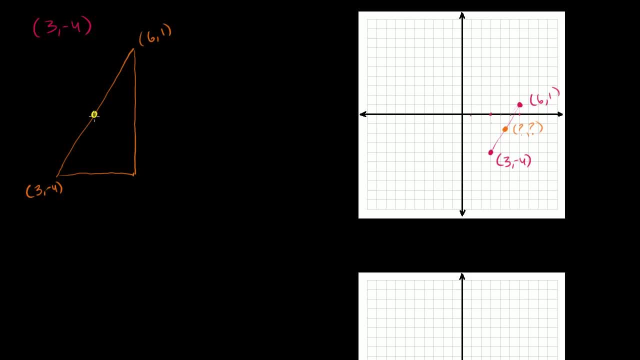 And we're looking at the point 6, comma 1.. And we're looking for the point that is smack dab in between those two points. What are its coordinates? It seems very hard at first, But it's easy when you think about it in terms of just the. 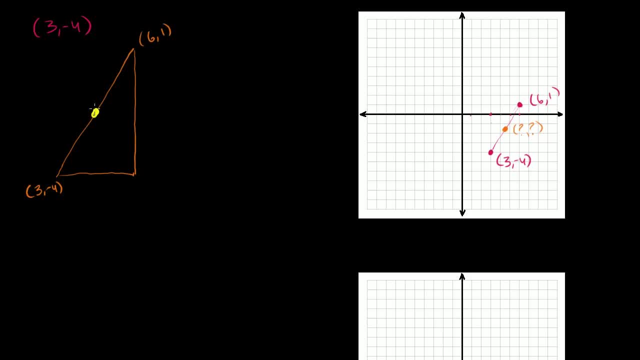 x and the y coordinates. What's this guy's x-coordinate going to be? This line out here represents x is equal to 6.. This over here represents x is equal to 6.. This over here represents x is equal to 3.. 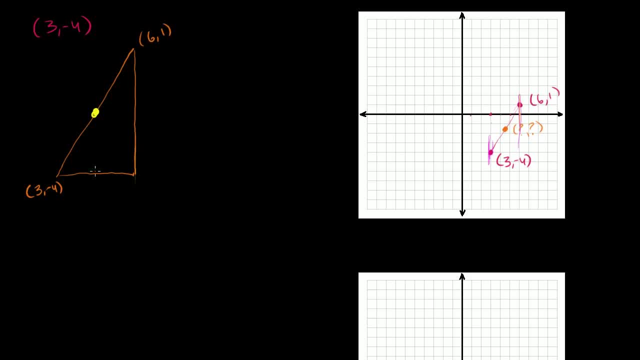 What will this guy's x-coordinate be? Well, he's going to be. His x-coordinate is going to be smack dab in between the two x-coordinates. This is x is equal to 3.. This is x equal to 6.. 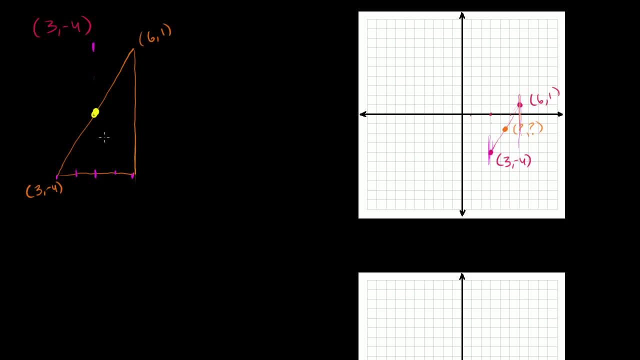 He's going to be right in between. This distance is going to be equal to that distance. His x-coordinate is going to be right in between the 3 and the 6.. So what do we call the number that's right in between the 3? 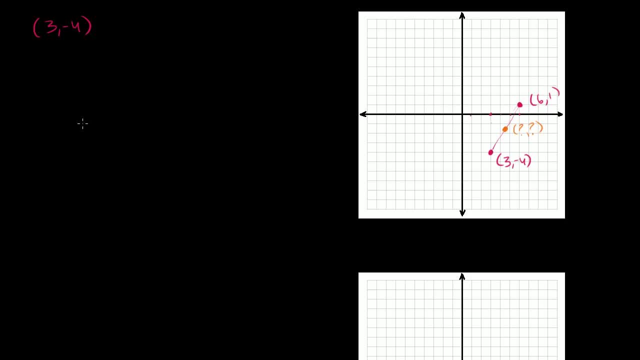 But you're going to see, it's actually one of the simplest things you'll learn in algebra and geometry. So let's say that this is my triangle, right there. This right here is the point 6, comma 1.. This down here is the point 3, comma negative 4.. 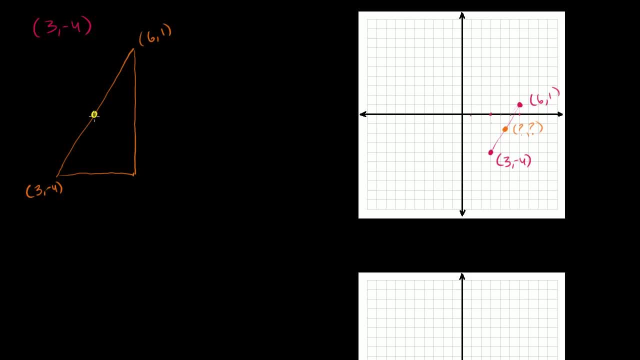 And we're looking at the point 6, comma 1.. And we're looking for the point that is smack dab in between those two points. What are its coordinates? It seems very hard at first, But it's easy when you think about it in terms of just the. 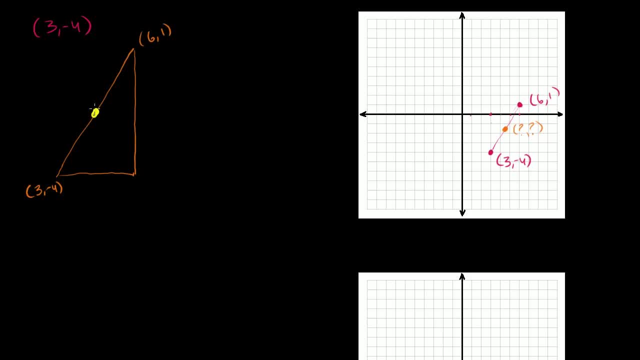 x and the y coordinates. What's this guy's x-coordinate going to be? This line out here represents x is equal to 6.. This over here represents x is equal to 6.. This over here represents x is equal to 3.. 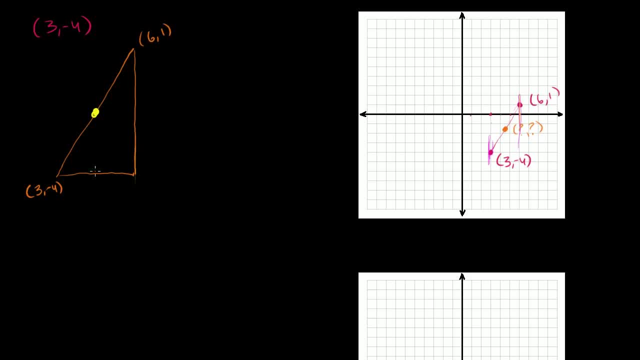 What will this guy's x-coordinate be? Well, he's going to be. His x-coordinate is going to be smack dab in between the two x-coordinates. This is x is equal to 3.. This is x equal to 6.. 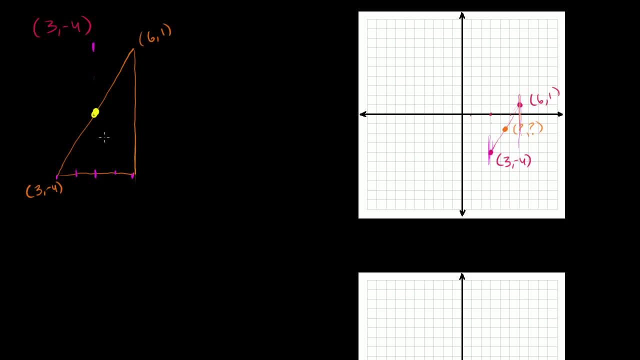 He's going to be right in between. This distance is going to be equal to that distance. His x-coordinate is going to be right in between the 3 and the 6.. So what do we call the number that's right in between the 3? 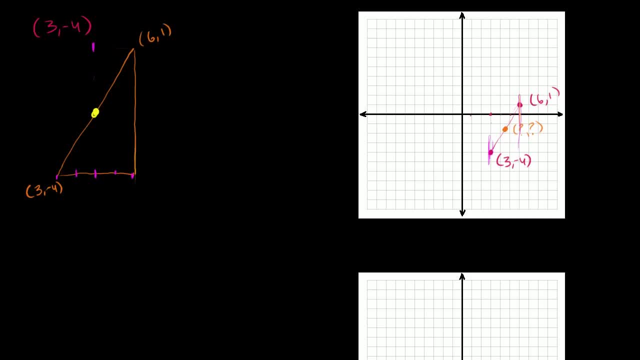 and the 6?? Well, we could even call that the midpoint, Or we could call it the mean, or the average, or however you want to talk about it. We just want to know what's the average of 3 and 6.. So, to figure out this point, the point halfway between 3. 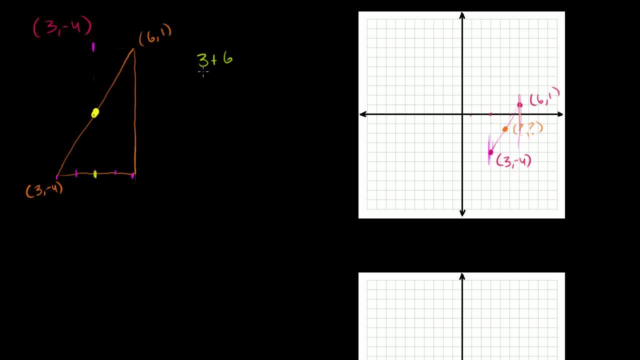 and 6, you literally just figure out 3 plus 6 over 2, which is equal to 4.5.. So this x-coordinate is going to be 4.5.. Let me draw that on this graph: 1,, 2,, 3,, 4.5. 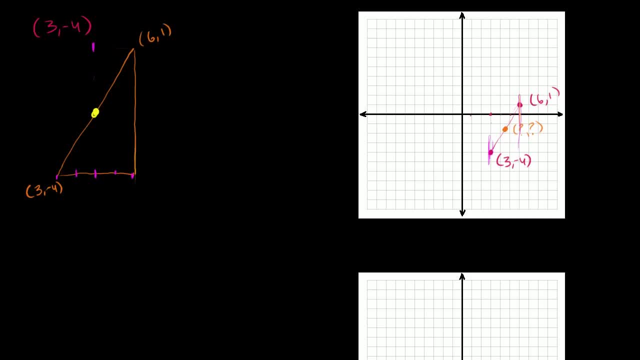 and the 6?? Well, we could even call that the midpoint, Or we could call it the mean, or the average, or however you want to talk about it. We just want to know what's the average of 3 and 6.. So, to figure out this point, the point halfway between 3. 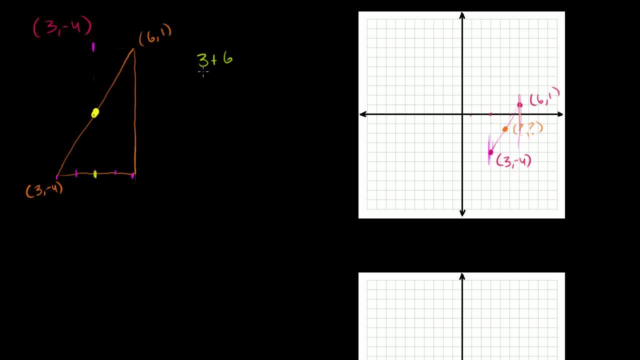 and 6, you literally just figure out 3 plus 6 over 2, which is equal to 4.5.. So this x-coordinate is going to be 4.5.. Let me draw that on this graph: 1,, 2,, 3,, 4.5. 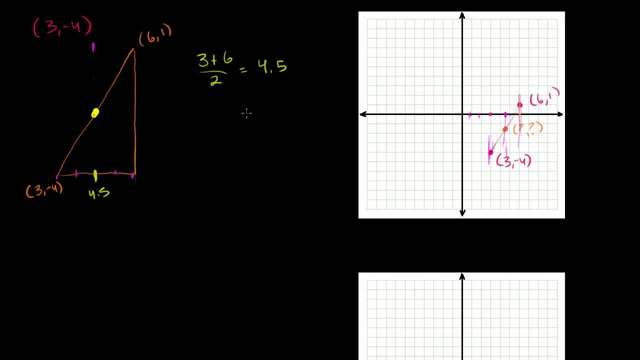 And you see it's smack dab in between. That's its x-coordinate. Now, by the exact same logic, this guy's y-coordinate is going to be 6.5.. Right, It's smack dab between. y is equal to negative 4 and y is. 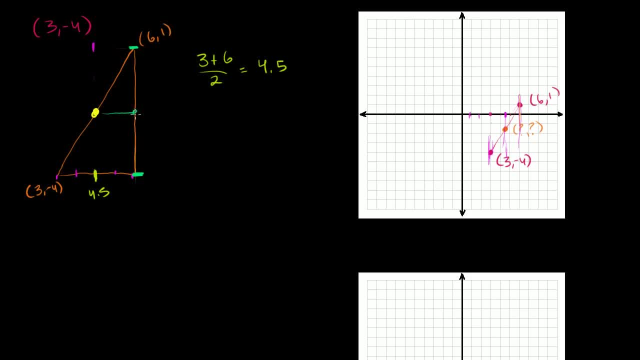 equal to 1.. It's just going to be right in between those. So this is the x, right there. The y-coordinate is just going to be right in between. y is equal to negative 4 and y is equal to 1.. So you just take the average. 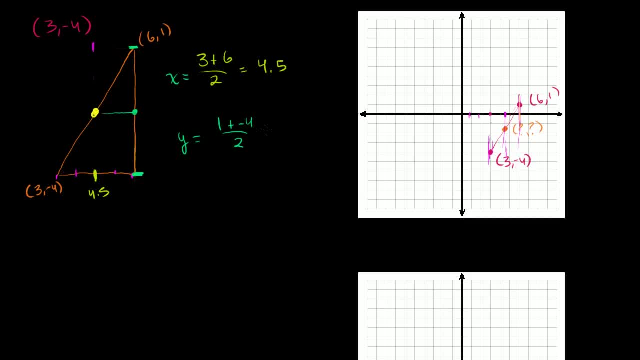 1 plus negative 4 over 2.. That's equal to negative 3 over 2.. Or you could say negative 1.5. So you go down 1.5. It is literally right there. So just like that, you literally take the average of. 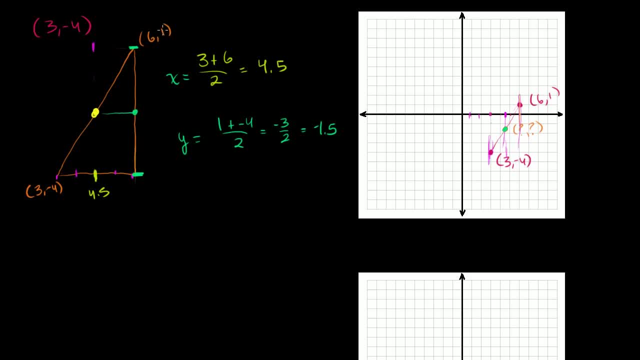 the x's. take the average of the y's, or maybe I should say the mean, to be a little bit more specific, a mean of only two points, and you will get the midpoint of those two points, the point that's equidistant from both of them. 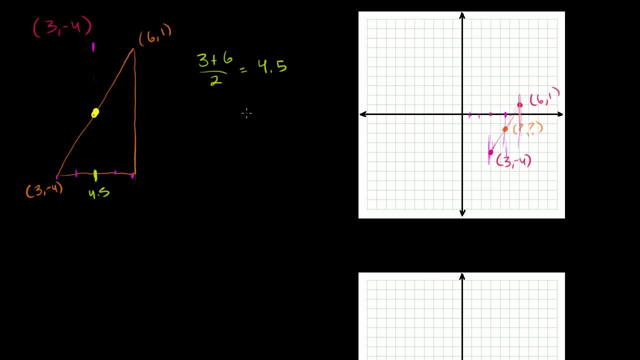 And you see it's smack dab in between. That's its x-coordinate. Now, by the exact same logic, this guy's y-coordinate is going to be smack dab between. y is equal to negative 4 and y is equal to 1.. 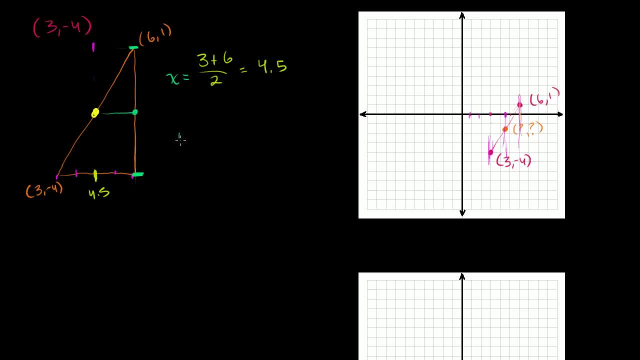 It's just going to be right in between those. So this is the x right there. The y-coordinate is just going to be right in between. y is equal to negative 4 and y is equal to 1.. So you just take the average. 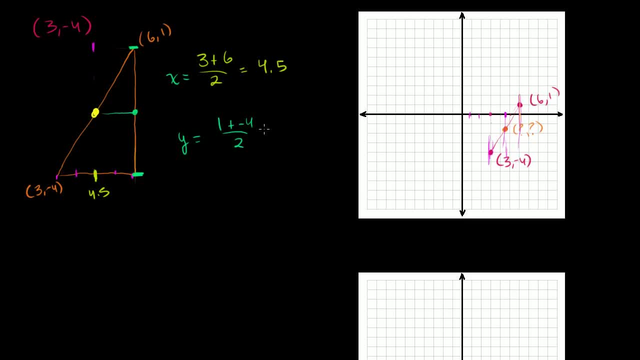 1 plus negative 4 over 2.. That's equal to negative 3 over 2.. Or you could say negative 1.5.. So you go down 1.5. It is literally right there. So just like that, you literally take the average of the x's. take the. 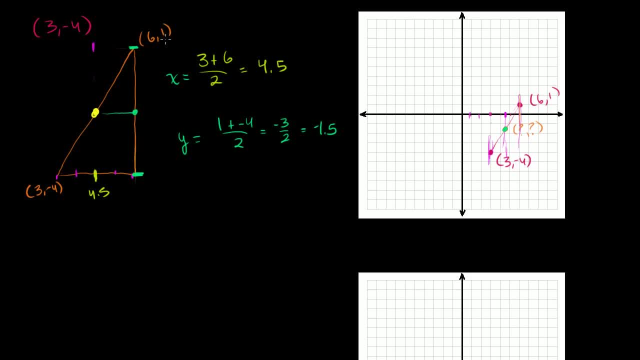 average of the y's, or maybe I should say the mean, to be a little bit more specific, a mean of only two points, and you will get the midpoint of those two points, the point that's equidistant from both of them. 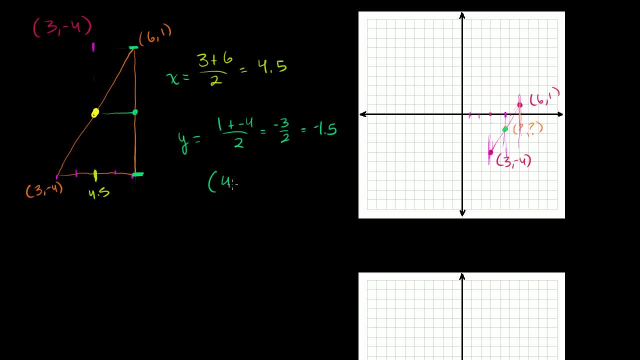 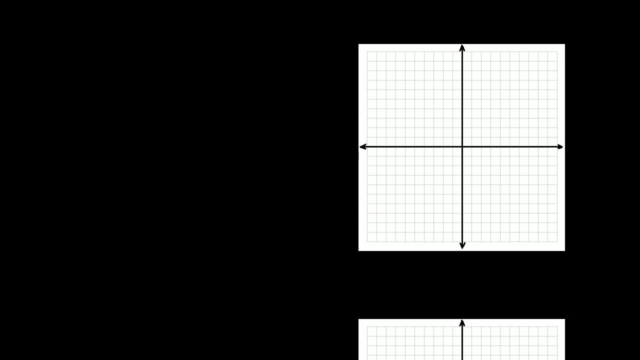 It's the midpoint of the line that connects them. So the coordinates are 4.5 comma negative 1.5.. Let's do a couple more of these. These actually, you're going to find are very, very straightforward, But just to visualize it, let me graph it. 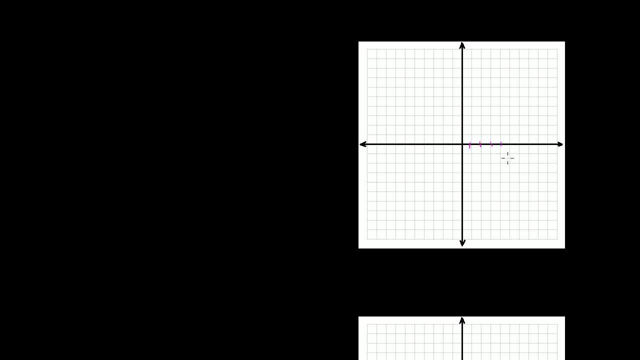 Let's say I have the point 4, negative 5.. So 1,, 2,, 3,, 4, and then go down 5.. 1,, 2,, 3,, 4,, 5.. So that's 4, negative 5.. 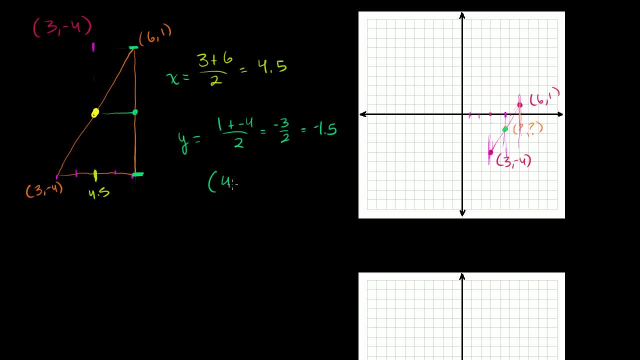 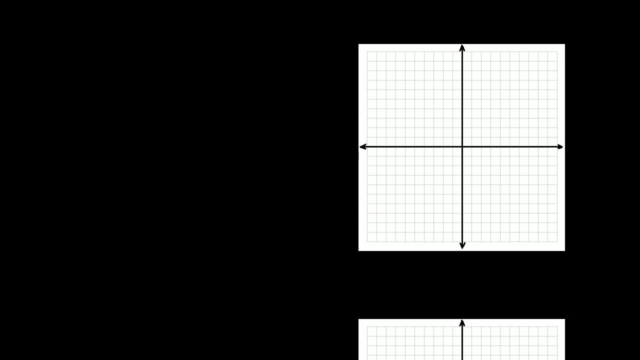 It's the midpoint of the line that connects them. So the coordinates are 4.5 comma negative 1.5.. Let's do a couple more of these. These actually, you're going to find are very, very straightforward, But just to visualize it, let me graph it. 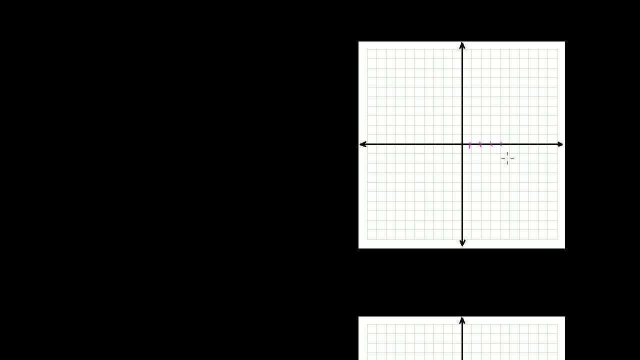 Let's say I have the point 4, negative 5.. So 1,, 2,, 3,, 4, and then go down 5.. 1,, 2,, 3,, 4,, 5.. So that's 4, negative 5.. 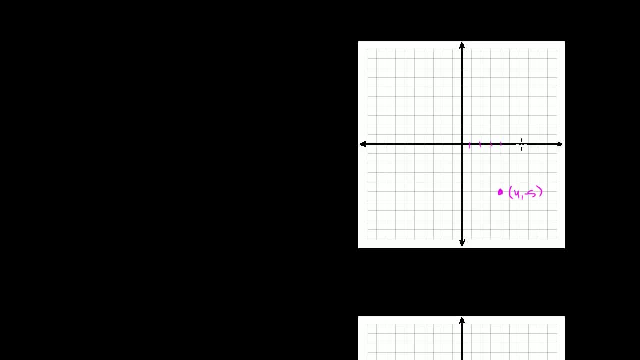 And I have the point 8, comma 2.. So 1,, 2,, 3,, 4,, 5,, 6,, 7,, 8 comma 2.. So what is the coordinate of the midpoint of these two points, the point that is smack dab in between them? 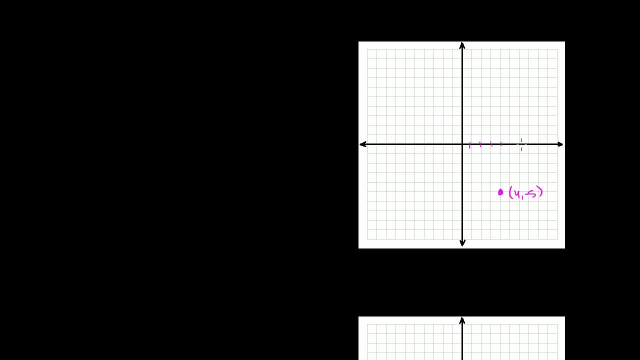 And I have the point 8, comma 2.. So 1,, 2,, 3,, 4,, 5,, 6,, 7,, 8 comma 2.. So what is the coordinate of the midpoint of these two points, the point that is smack dab in between them? 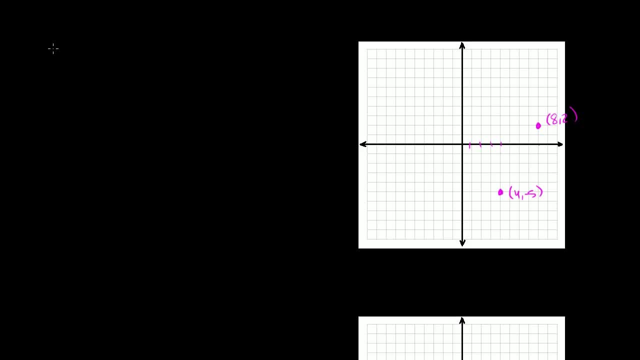 Well, we just average the x's, average the y's. So the midpoint, The midpoint is going to be: the x values are 8 and 4.. So it's going to be 8 plus 4 over 2.. And the y value is going to be: well, we have a 2 and a negative 5.. 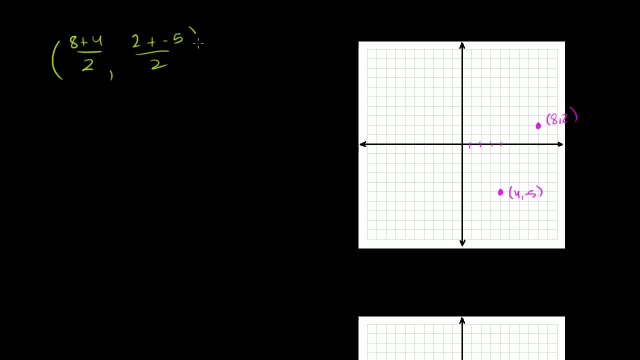 So you get 2 plus negative 5 over 2.. And what is this equal to? This is 12 over 2,, which is 6 comma. 2 minus 5 is negative 3.. Negative 3 over 2 is negative 1.5.. 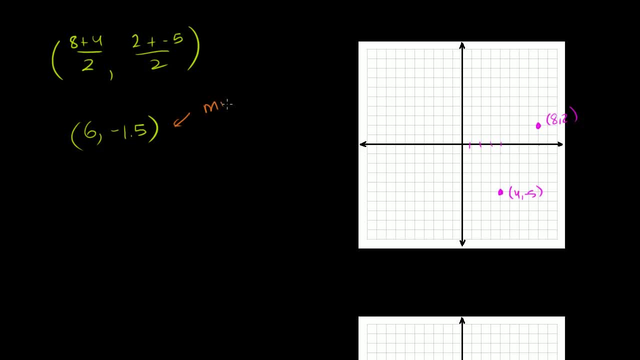 So that, right, there is the midpoint. It is the midpoint. You literally just average the x's and average the y's or find their mean. So let's graph it, just to make sure it looks like the midpoint: 6, negative: 5.. 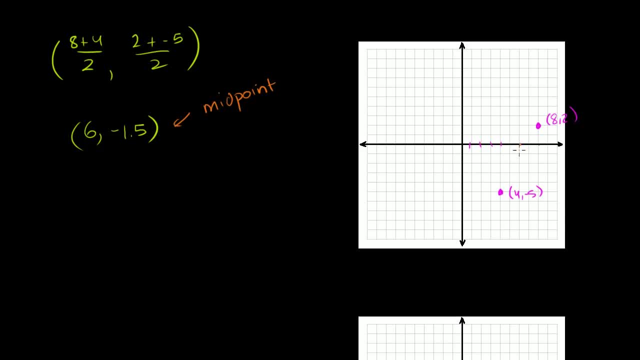 1, 2,, 3,, 4, 5, 6.. Negative 1.5.. Negative 1, negative 1.5.. Yeah, looks pretty good. It looks like it's equidistant from this point. 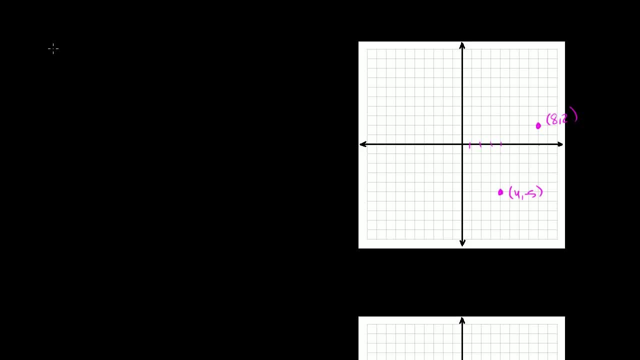 Well, we just average the x's, average the y's, So the midpoint 8 is going to be. the x values are 8 and 4.. So it's going to be 8 plus 4 over 2.. And the y value is going to be. well, we have a 2 and a. 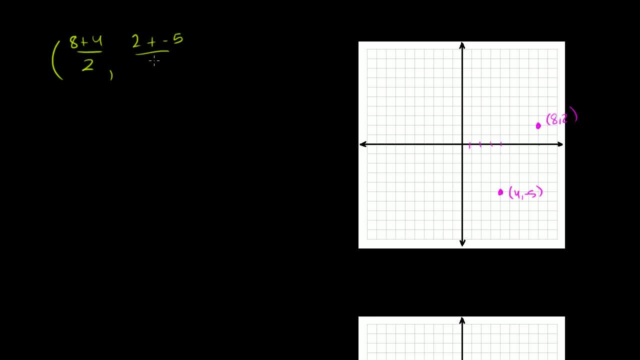 negative 5.. So you get 2 plus negative 5 over 2.. And what is this equal to? This is 12 over 2,, which is 6 comma. 2 minus 5 is negative 3.. Negative 3 over 2 is negative 1.5.. 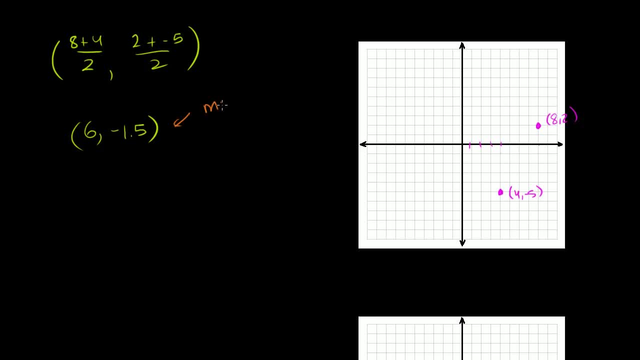 So that right there is the midpoint. You literally just average the x's and average the y's or find their mean. So let's graph it, just to make sure it looks like the midpoint: 6, negative, 5.. 1,, 2,, 3,, 4,, 5, 6.. 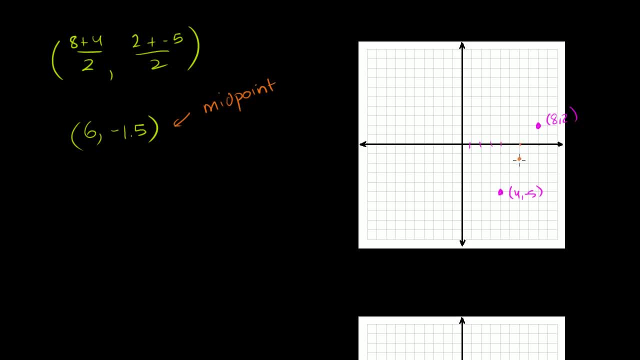 Negative 1.5.. Negative 1, negative 1.5.. Yeah, looks pretty good. It looks like it's equidistant from this point and that point up there. Now, that's all you have to remember. Average the x, or take the mean of the x, or find the x, that's. 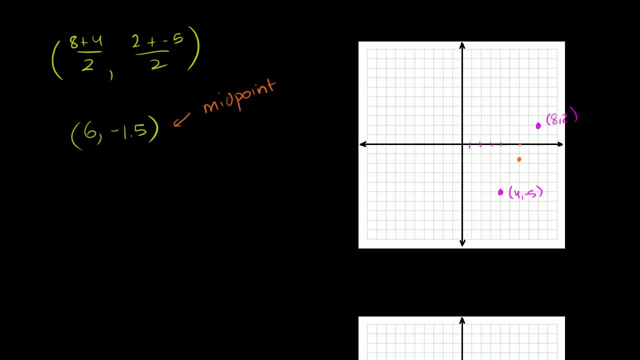 right in between the two, Average the y's. You've got the midpoint. What I'm going to show you now is what's in many textbooks. They'll write: oh, if I have the point x1,, y1,, and then I 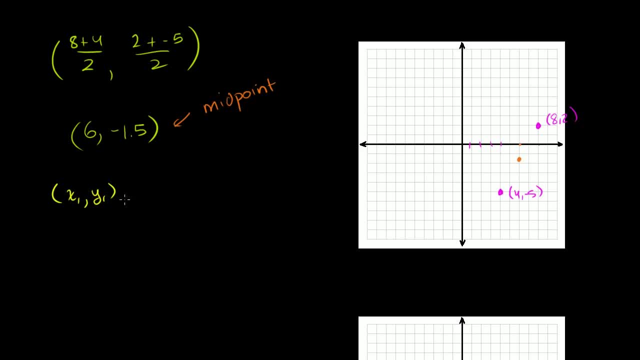 have the point. actually I'll just stick in yellow. it's kind of painful to switch colors all the time. and then I have the point x2, y2,. many books will give you something called the midpoint formula, which, once again, I think is kind of silly. 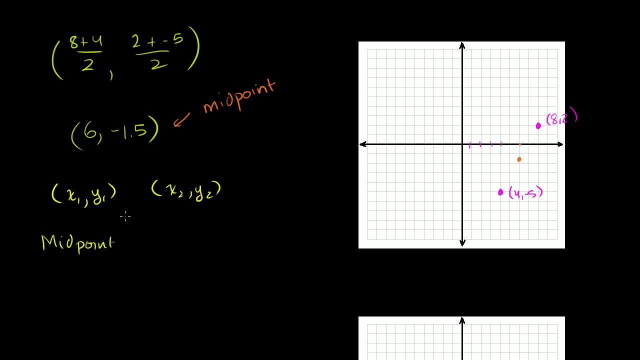 to memorize. Just remember you just average: find the x in between, find the y in between. So midpoint, formula, Formula. What they'll really say is the midpoint, so maybe we'll say the midpoint x, or maybe I'll call it this way: 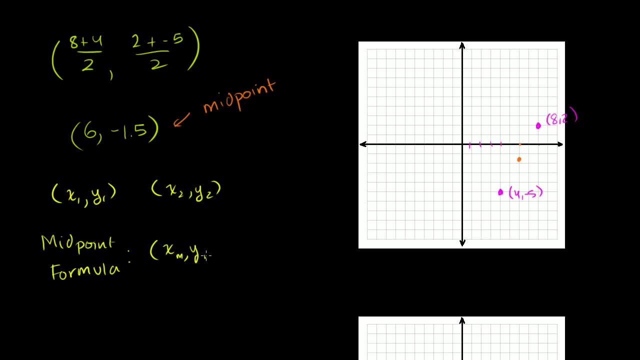 I'm just making up notation- The x midpoint and the y midpoint is going to be equal to- and they'll give you this formula: x1 plus x2 over 2, and then y1 plus y2 over 2, and it looks like something you have. 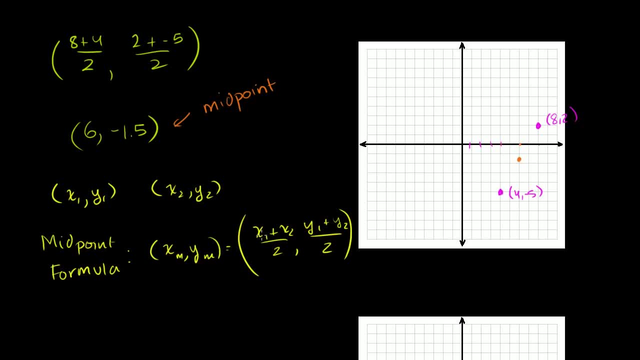 to memorize. But all you have to say is: look, that's just the average or the mean of these two. This is just the average or the mean of these two numbers. I'm just saying I'm adding the two together, dividing by 2,.